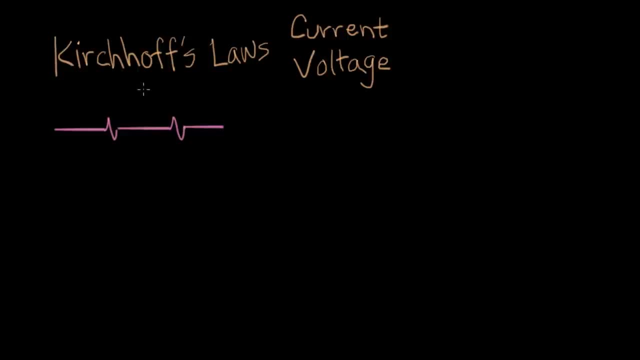 The idea of Kirchhoff's Laws. these are basically common sense laws that we can derive from looking at simple circuits, and in this video we're gonna work out Kirchhoff's Current Law. Let's take a look at these series: resistors here. 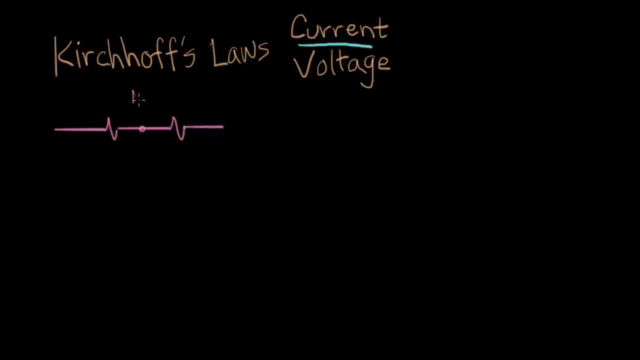 There's a connection point right there and that's called a node, a junction, And one of the things we know is that when we put current through this, let's say we put a current through here and we know that current is flowing charge. 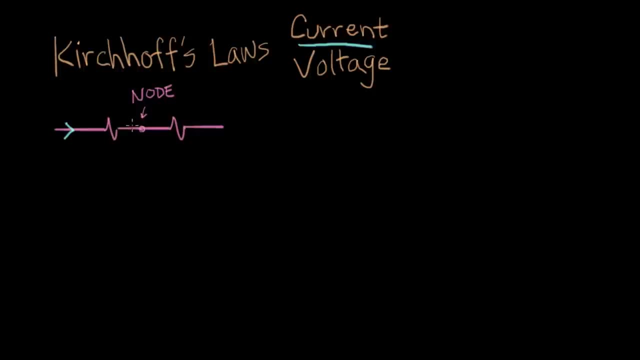 so we know that the charge does not collect anywhere. so that means it comes out of this resistor and flows into the node and then goes across and it comes out. It comes out on this side. All the current that comes in comes out. 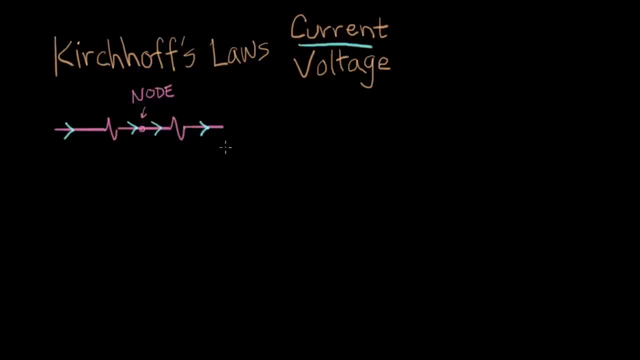 That's something we know, That's the conservation of charge, and we know that the charge does not pile up anywhere. We'll call this current I1, and we'll call this current I2.. And we know we can just write right away: I1 equals I2.. 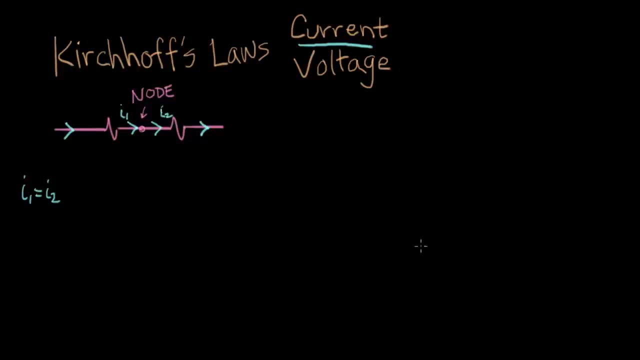 That seems pretty clear from our argument about, about, about the current. That seems pretty clear from our argument about charge. Now let me add something else here. We'll add another resistor to our node like that And this: now there's gonna be some current going this way. 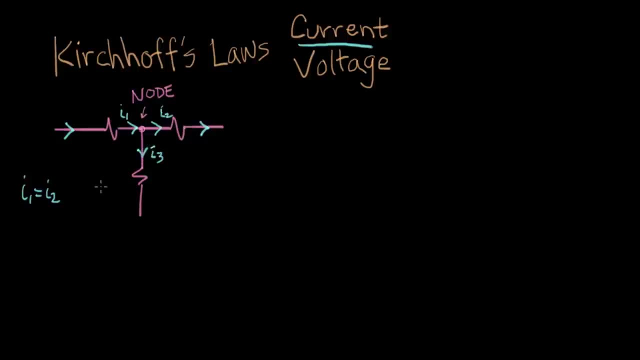 Let's call that I3.. And now this doesn't work anymore. This I1 and I2 are not necessarily the same, But what we do know is any current that goes in has to come out of this node. So we can say that I1 equals I2 plus I3.. 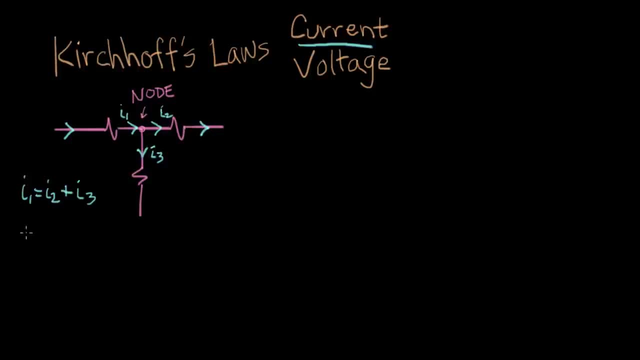 That seems pretty clear, Pretty reasonable And, in general, what we have here is, if we take all the current flowing in, it equals all the current flowing out, And that's that's Kirchhoff's current law. That's one way to say it. 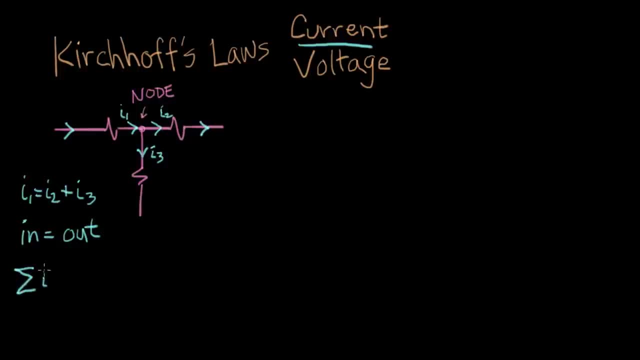 In. in mathematical notation we would say I in the summation of currents going in. that's the summation sign, is the summation of I in. That's one way to say it. That's one expression of Kirchhoff's current law. 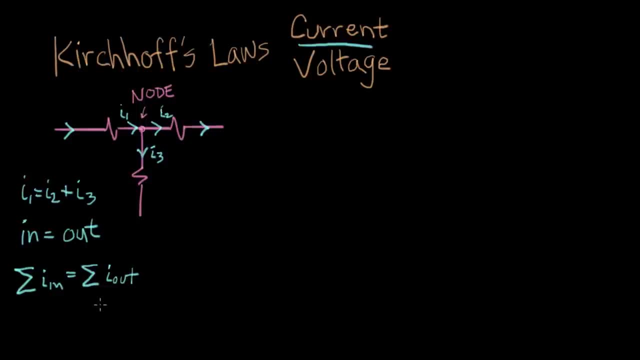 That's one expression of Kirchhoff's current law. That's one expression of Kirchhoff's current law. So now I I wanna generalize, I wanna generalize this a little bit. Let's let's say we have a node. 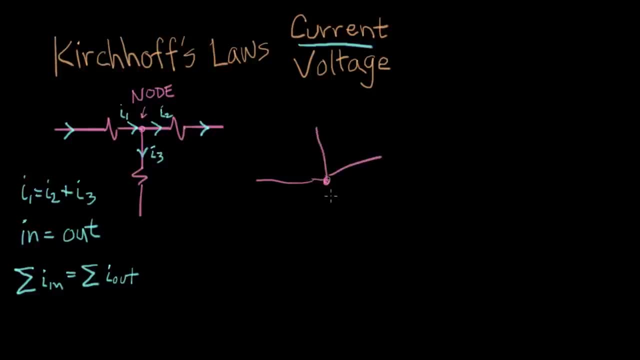 and we have some wires going into it. Here's some wires connected up to a node And there's current going into each one. I'm gonna define the current arrows. This, this is this- looks a little odd, but it's okay to do. 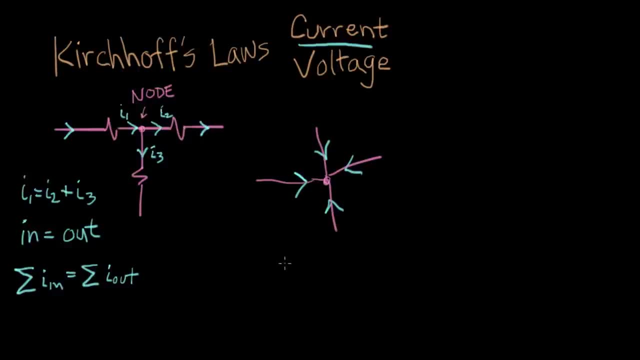 All going in, And what Kirchhoff's current law says is that the sum of the currents going into that node has to be equal to zero. Let's, let's work out how that works. Let's say: this is one amp. 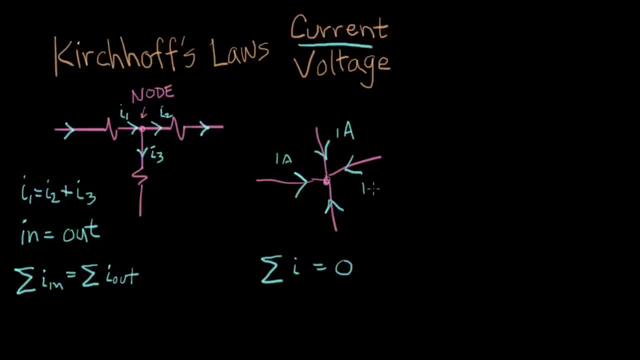 and this is one amp and this is one amp. And the question is: what is this one? What's that current there? If I use my, if my current law expressed this way, it says that one plus one plus one plus I. 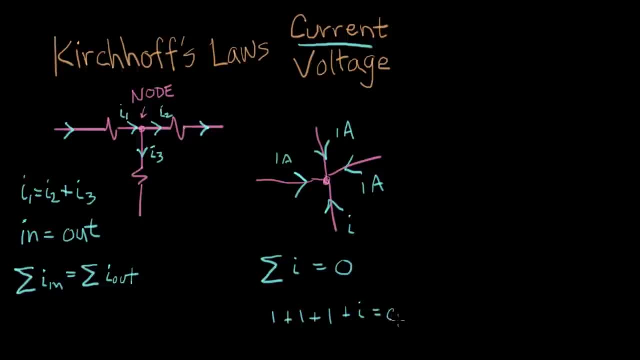 whatever this I here has to equal zero And what that says is that I equals minus three. So that says minus three amps flowing in is the same exact thing as plus three amps flowing out. So one amp, one amp. one amp comes in, three amperes flows in. 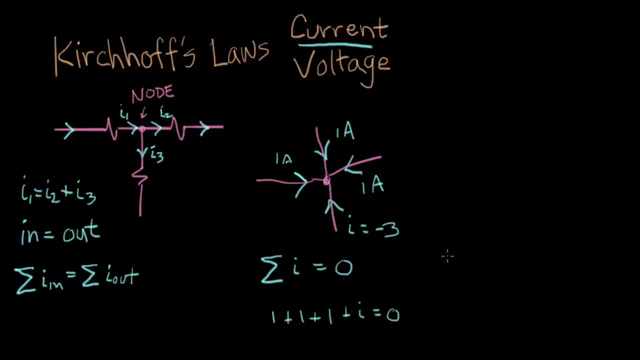 So one amp, one amp. one amp comes in three amperes flows in, Then two amps, two amps coming in, three amperes flows out. Another way we could do it, equally valid. This is just three ways to say exactly the same thing. 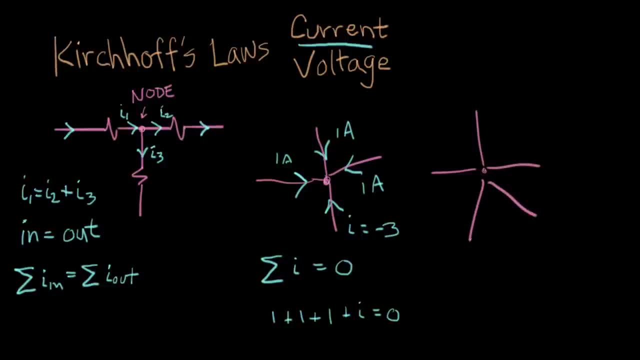 I have a bunch of wires going to a junction like this and this time I define the currents going out. Let's say I define them all going out And the same thing works: Sum of the currents. I'll go back over here, I'll write in. 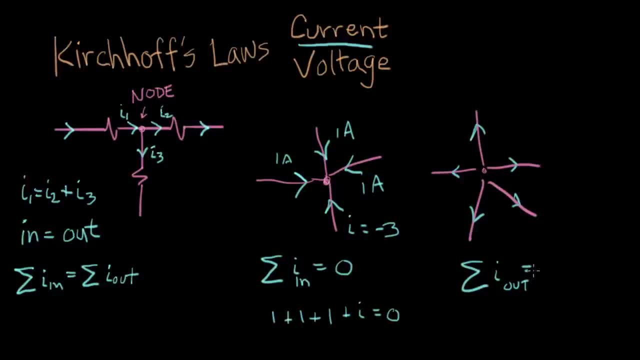 all the currents going in, That has to equal zero as well. And you can do the same exercise If I make all these one amp and ask: what is this one here? what is I here? Outgoing current, it's one plus one plus one plus one. 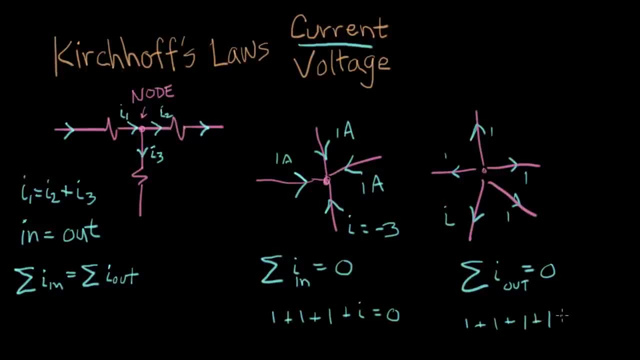 Those are the four that I know and those are the ones going out. So what's the last one going out? It has to equal zero. The last one has to be minus four equals zero. So this is a current of minus four amperes.